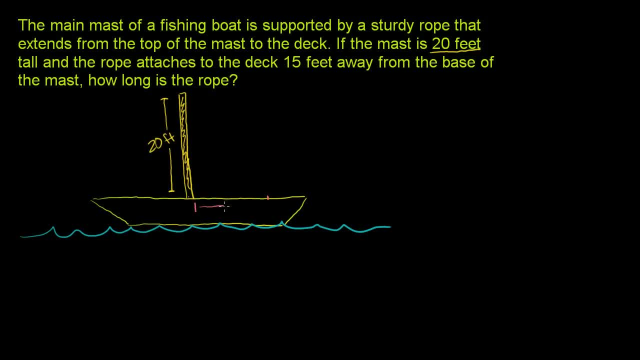 Might be about that distance right there. Let me mark that This distance right there is 15 feet, And the rope attaches right here, From the top of the mast all the way to that base. So the rope goes like that, And then they ask us how long is the rope? 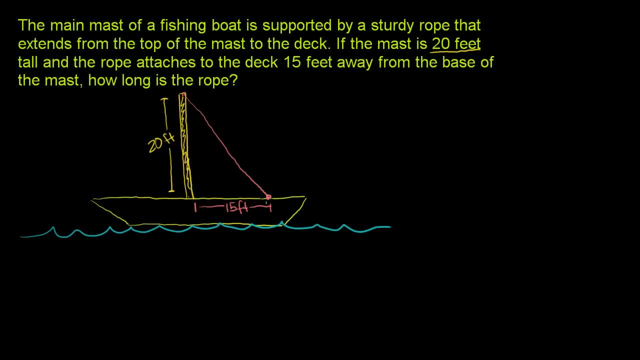 So there's a few things you might realize. We're dealing with a triangle here, And it's not any triangle. We're assuming that the mast goes straight up and that the the deck is straight left and right, So this is a right triangle. 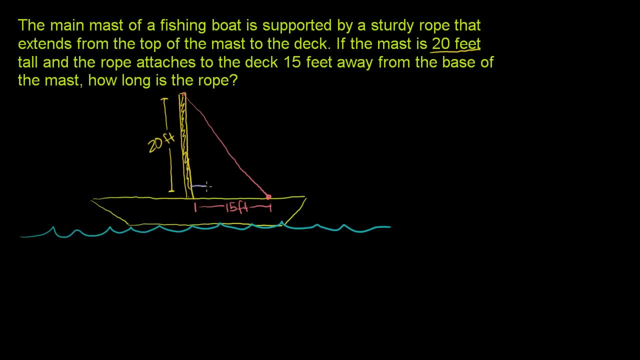 This is a 90 degree angle right here. This is a right triangle, And we know that if we know two sides of a right triangle, we can always figure out the third side of the right triangle using the Pythagorean theorem, And all that tells us is that the square 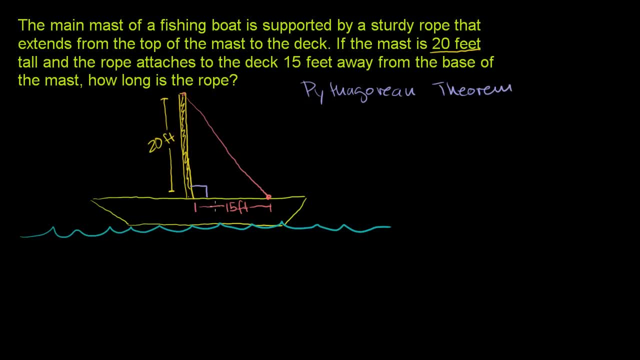 the sum of the squares of the shorter sides of the triangle are going to be equal to The square of the longer side, And that longer side is called the hypotenuse. And in this case- well, in all cases- the hypotenuse is the side opposite the 90 degree angle. 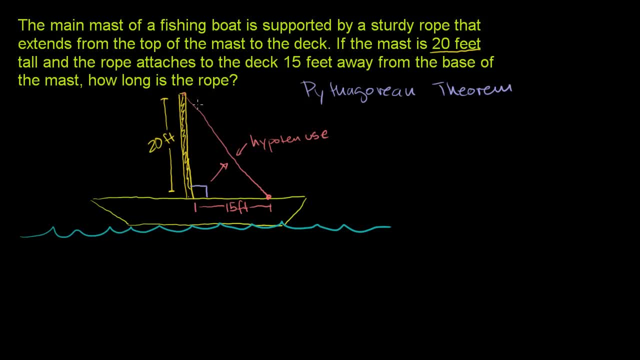 It's always going to be the longest side of our right triangle. So we need to figure out the hypotenuse here. We know the lengths of the two shorter sides, So we can see that if we take 15 squared, that's one of the shorter sides. 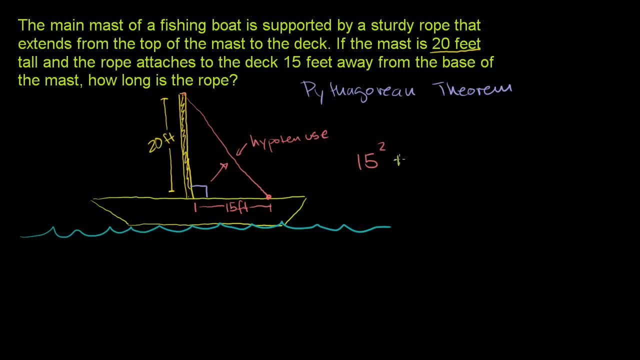 I'm squaring it And then add that to the square of the other shorter side, to 20 feet squared. And when I say the shorter side I mean relative to the hypotenuse. The hypotenuse will always be the longest side. 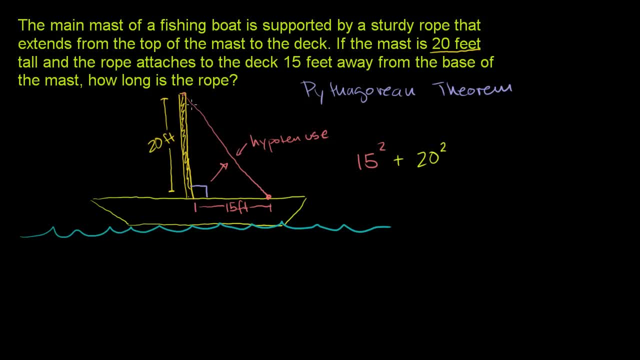 That is going to be equal to, Let's say, the hypotenuse is in green, just so we get our color coding. nice, That is going to be equal to the rope squared or the length of the rope. So let's call this distance right here. r. 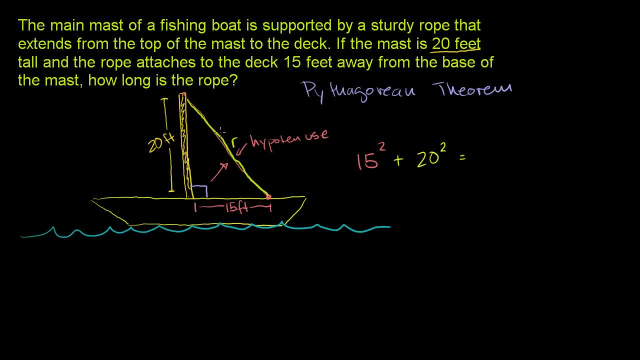 r for rope. Let me do it a little bit neater than that. r for rope Is the length of the rope. So 15 squared plus 20 squared is going to be equal to r squared. And what's 15 squared?